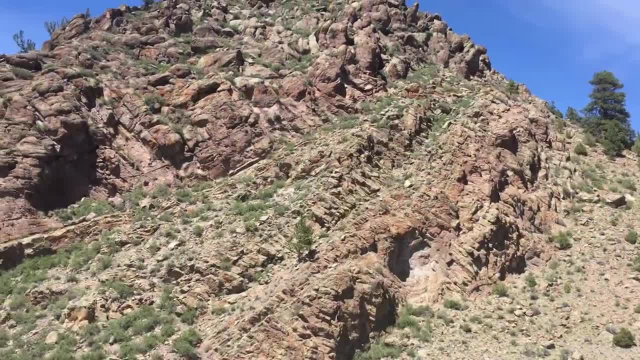 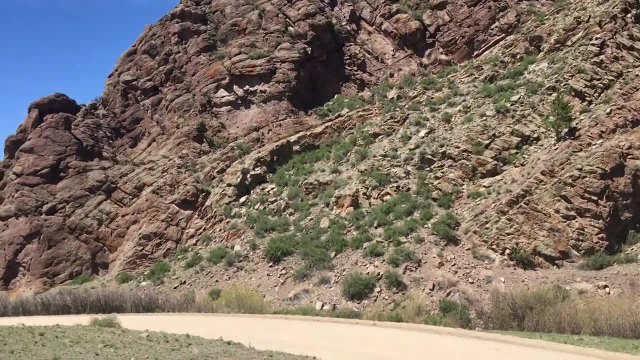 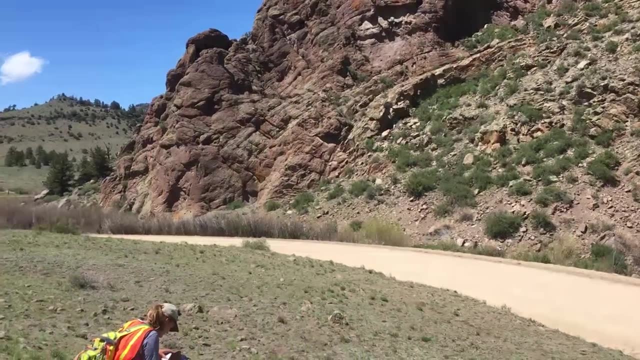 and some focus on structural geology, the unraveling, the twists and turns and the folds that many areas go through, recorded in present rock positions. And in doing so we can also focus on distant past history of a location and unravel Earth's tales with its peaceful, tranquil times, occasionally punctuated with episodes of drama and terror. 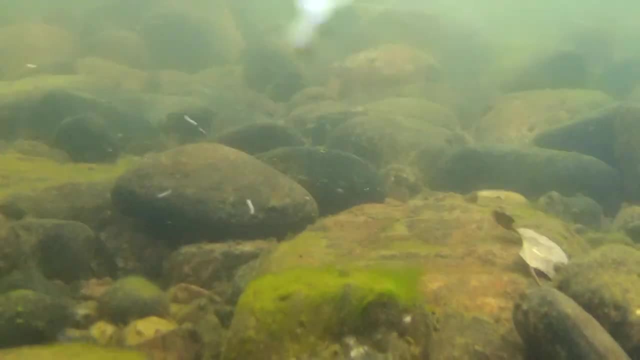 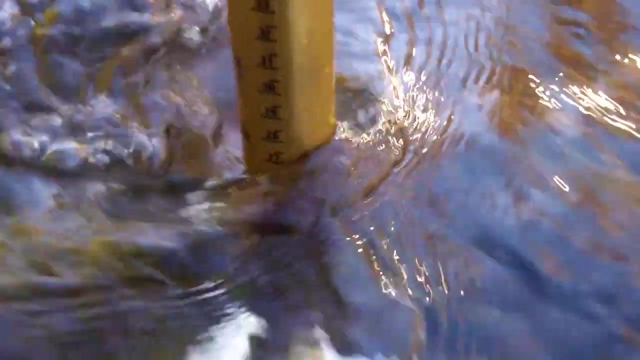 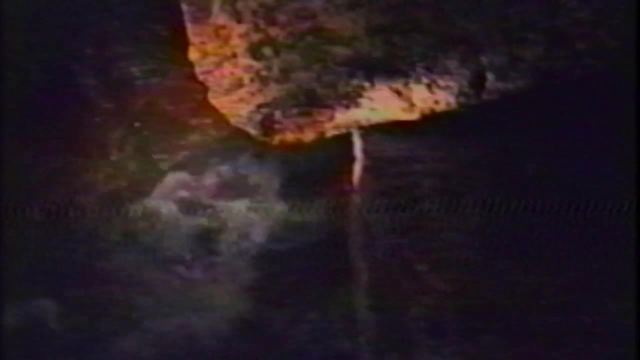 Our rocks tell us stories of a biosphere that has been sustained by the waters of life, upon which we also focus. Hydrogeology is the study of Earth's water above and below ground, and I can say without a moment's hesitation that this will be an important field for the rest of your lives. 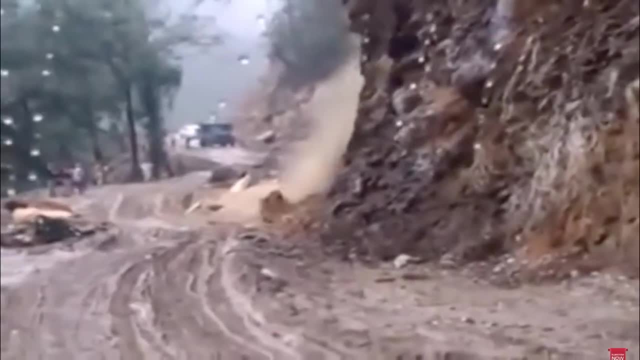 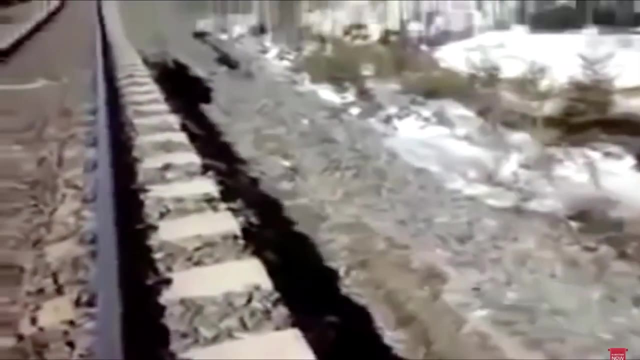 And I hope your lives are long, which is helped by avoiding natural disasters, which is what we focus on in engineering, geology: the identification and mitigation of risks to get lives out of harm's way and avoid damage and recover our infrastructure. 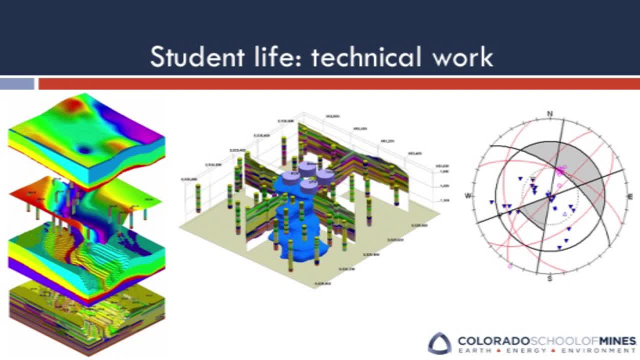 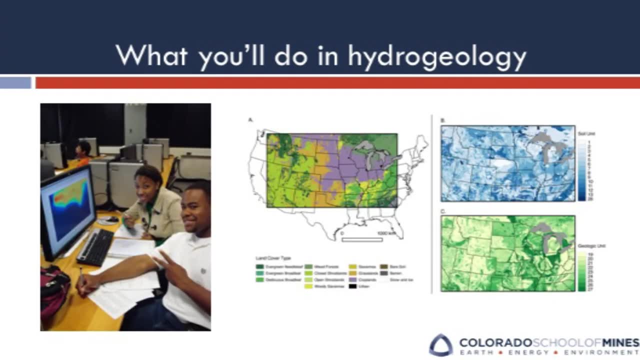 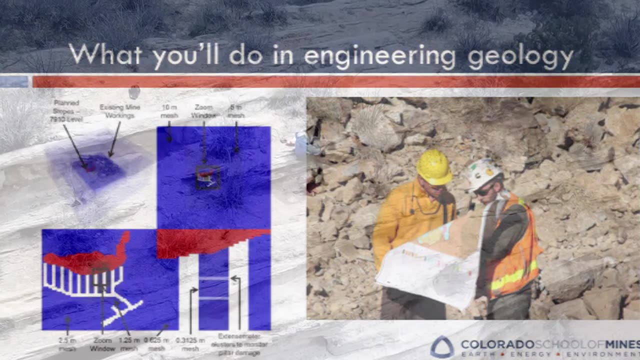 We work with computers and the software that will best prepare our students to enter the workforce with competence And support our students' understanding of the concepts and mathematics to best utilize such tools. But we also maintain a focus on field exploration through our many field trips. 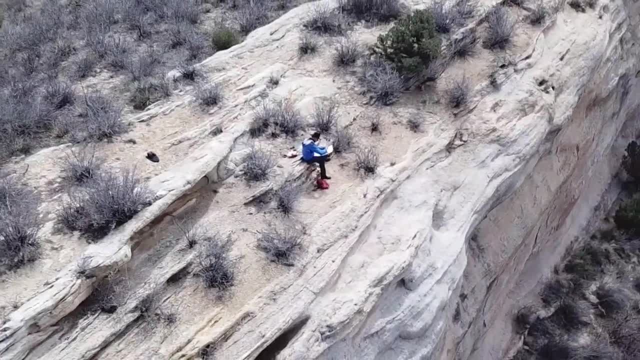 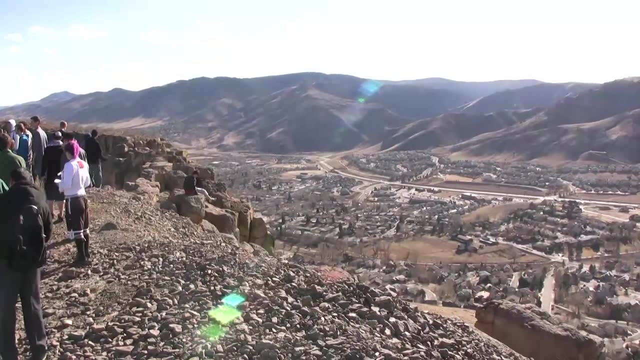 starting with the amazing geology right in our backyard, which I hope to personally take you on if you come here and take GEGN 101- Earth and Environmental Systems- with me. But as you continue in your studies, you will be stretching out to other parts of the state. 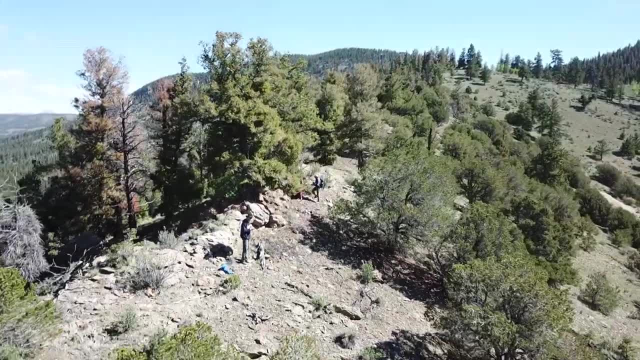 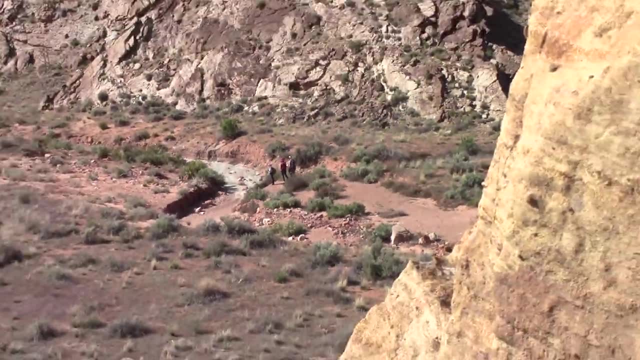 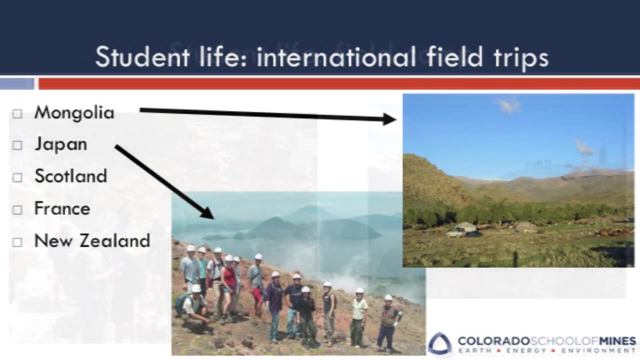 which I will have a hard time not swearing while describing the amazing diversity geologically available to us in the state of Colorado and so for the region that we explore, And we even take trips to explore locations around the world. Our students experience our top-rated six-week summer field camp between their junior and senior years. 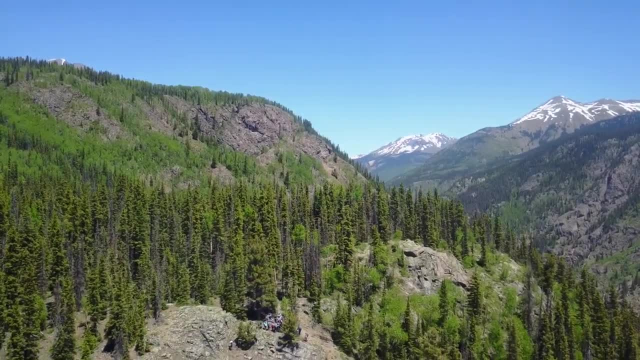 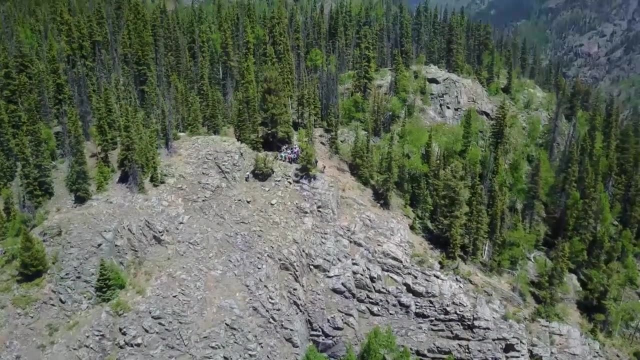 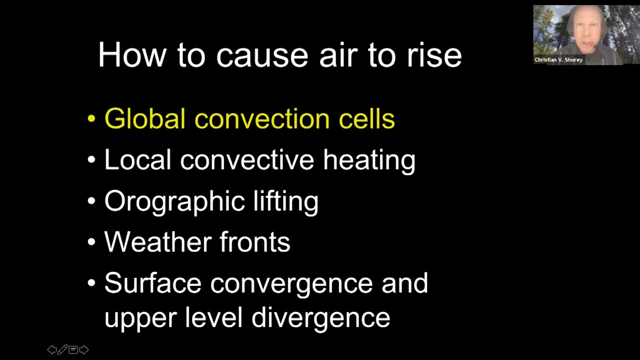 and transform from geology students to geologists in some of the best locales you can imagine for what we are looking at, all within relatively easy reach of our campus. We have even been able to weather remote teaching successfully with our technical resources and creative and competent staff and students.